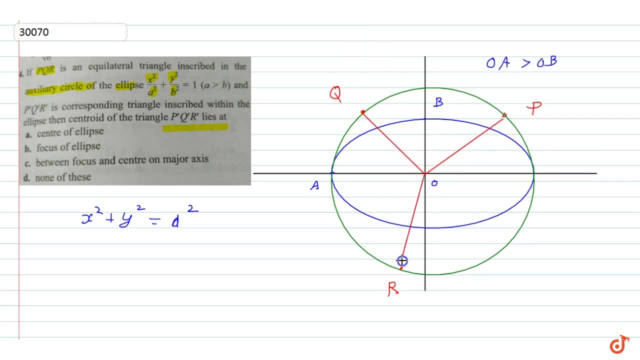 We know. So P, Q, R. Okay, These are our three points, And what will be our triangle? Our triangle. Let me join our triangle as well. So this is our triangle: P, Q, Q, R And P? R. Now, 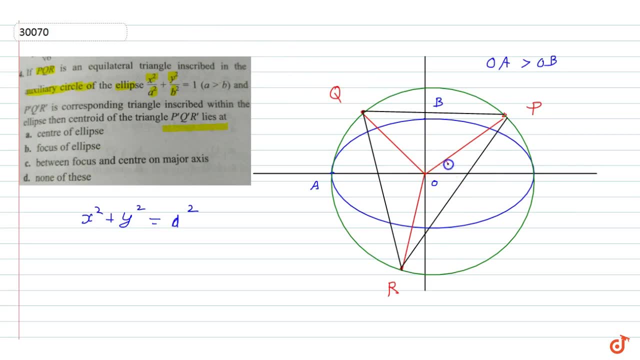 from here. let's say that. I say that the first point is P. This is at theta angle. Okay, This is at theta angle. So what will be the second angle? It will be at theta plus 120. Because this angle is also 120. And what will be this angle? This is also at 120.. So 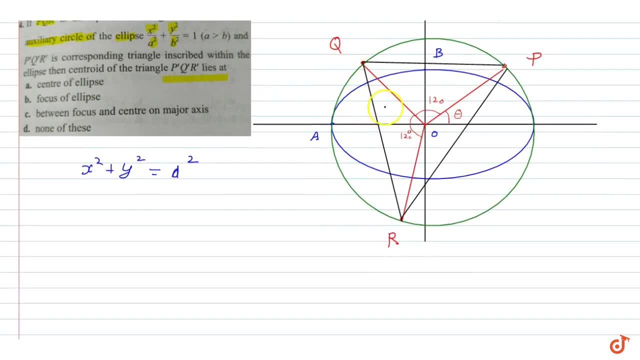 this means, if I see, then P Q R is equal to P, Q R is equal to P, Q R is equal to R, So this angle will be equal to P Q R. Now, P Q R can't be same, So enter it. 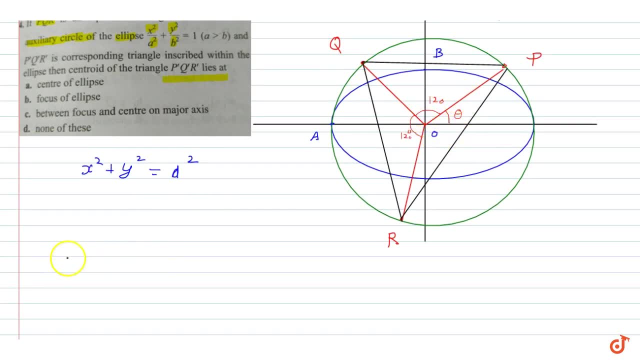 How is this triangle calculated If it's center? So what is the centroid of P Q R? It's E ray force. What is the centroid height of P Q R, Which is P Q R? So we can say, since 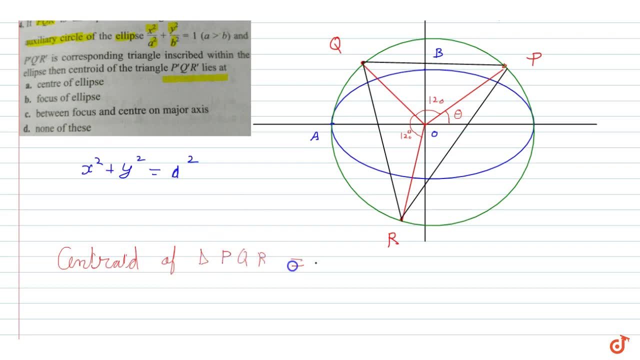 this is a equilateral triangle, then its centroid will be all same. The centroid will be the center. So from here, what is the centerhh? So, Cloid form, Centroid of Q, Q R. What "''an' Centroid Cl retrieved. So Centroid of P Q R is equal to what 0, 0 origin. Now, what is the? 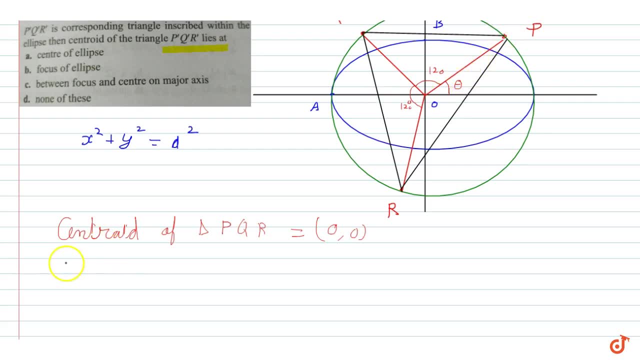 centroid. Well, here, if I call this centroid as a principleいく Book ofArchive, what will it become? This point will be A cos theta, so we will write its x-coordinate, so it will be A cos theta. then it will be A cos theta plus 120,, so it will be A cos theta plus 120, and then it will be plus A cos theta plus 240, upon which the value will be y3.. 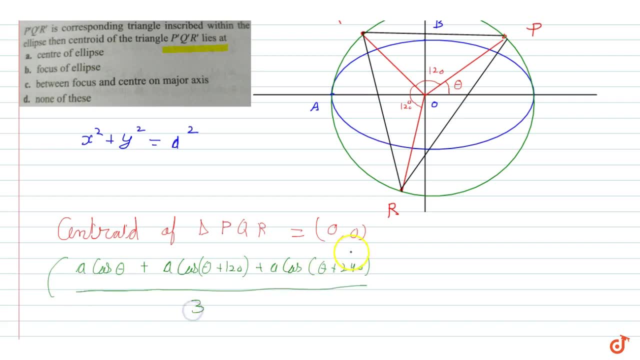 Similarly, if we write it for y, then it will be A sin theta plus 3,- sorry, A sin theta. then it will be plus A sin theta plus 120, then it will be plus A sin theta plus 240, theta plus 240. 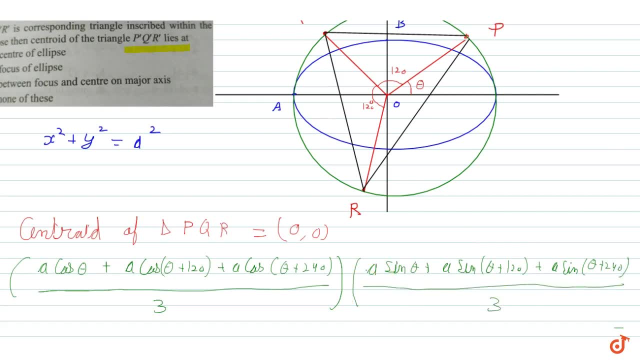 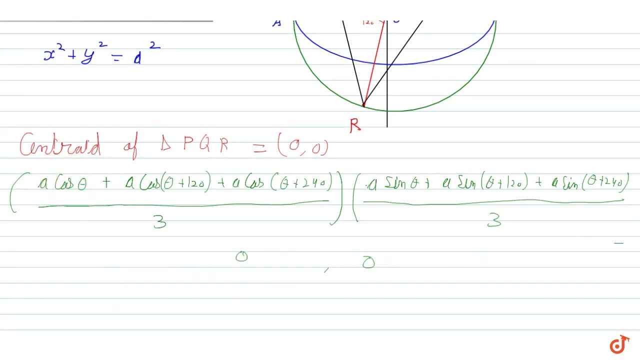 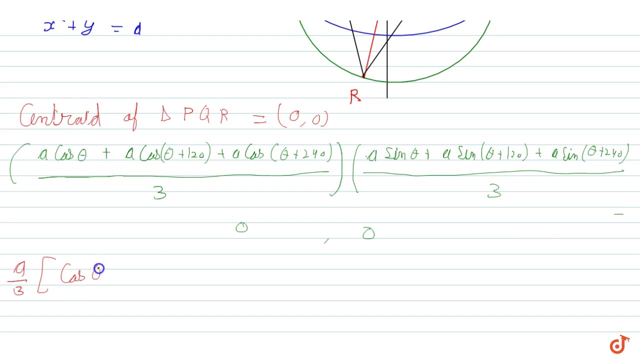 Upon which it will be y3, and this value will be equal to 0,. this is equal to 0, so it means if I take A common out of this, then the value will be A by 3 common. from here it will be A by 3 common, that cos theta plus cos theta plus 120 degree plus cos theta plus 240 degree. 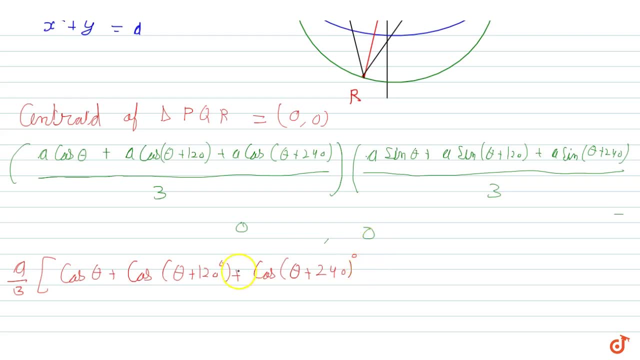 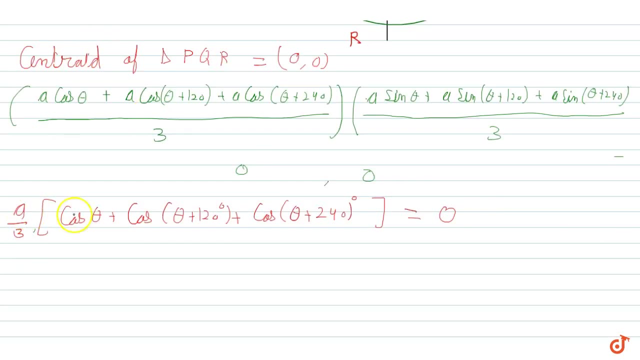 Okay, What will be this value? If we will look, we know this value: its equal to 0.. Now we have written it for x-coordinates. It mean that we know that A is our non-zero term Player discussion Now, similarly, similarly for sin also, what would it be? 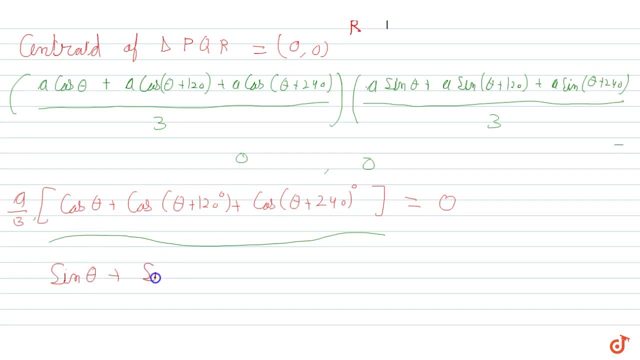 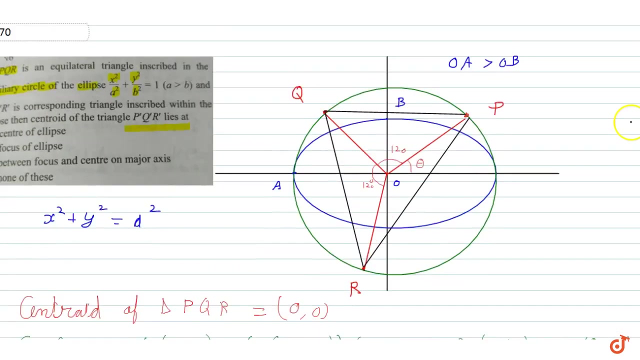 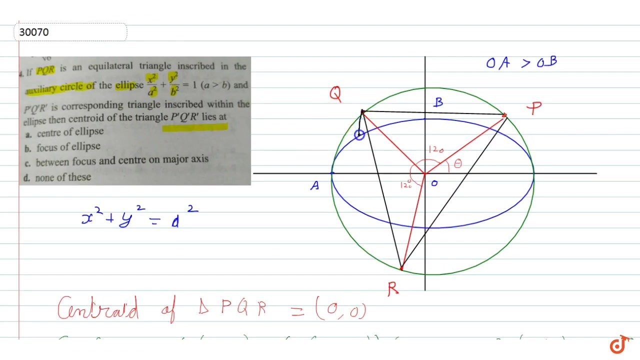 Sin theta plus Sin theta plus 120 degree, plus sin theta plus 240 degree, this will also be equal to 0. now, okay, now we will be given the corresponding point which is in the ellipse. if we see the corresponding point in the ellipse, then it will be this: 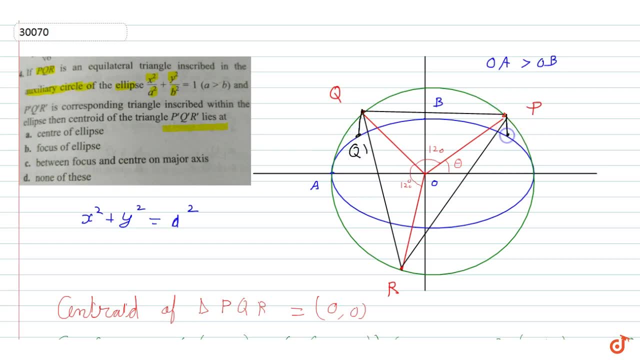 this point is q dash. if we see the corresponding point here, then this point is p dash, and if we see the corresponding point here, then this point is r dash. okay, so again, if we see, then we get to know that there is no change in the x coordinate. 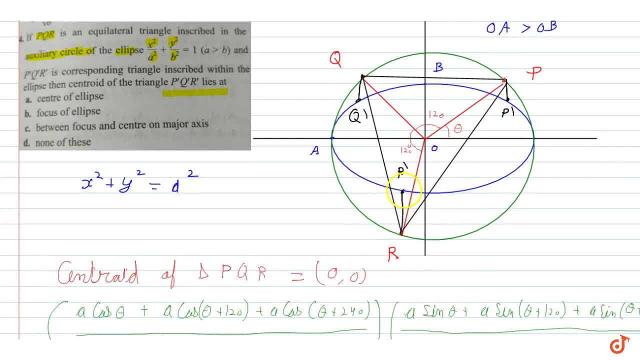 so if in the x coordinate, by doing this at this point, what is the same x coordinate, then our p dash, q dash and r dash triangle, its centroid will also be, its x coordinate will be 0, why? because if we see here, there is no change in x. 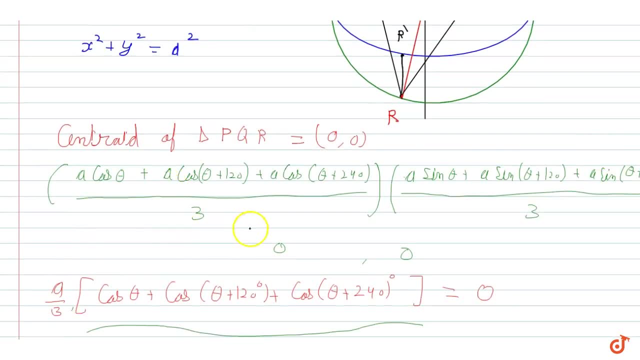 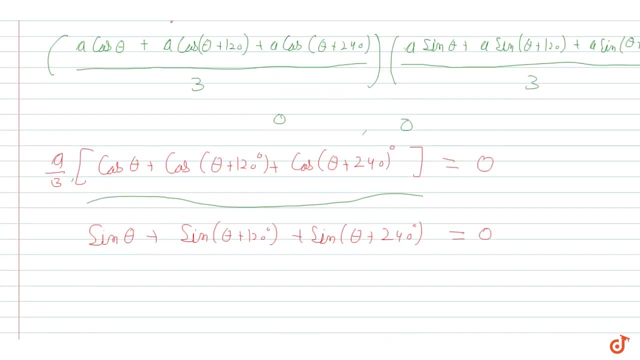 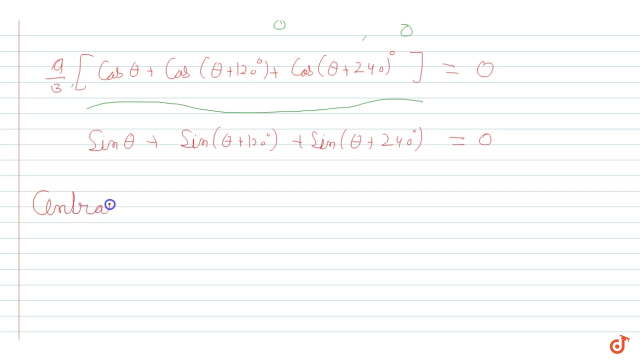 and we have already seen that the sum of x is 0. okay, and any point on this is a, cos theta, comma, b, sin theta, okay. so again, what we can say from here: centroid of centroid of what triangle? p dash, q dash, r dash, okay. so, as we know,